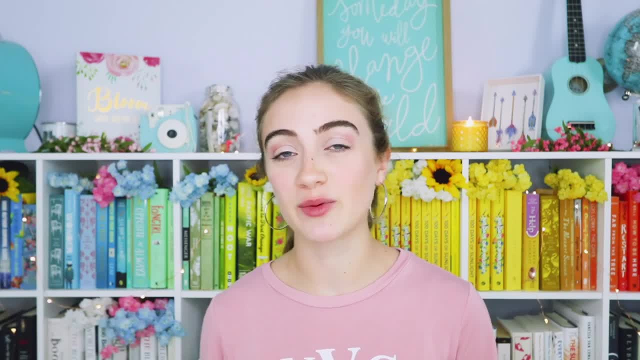 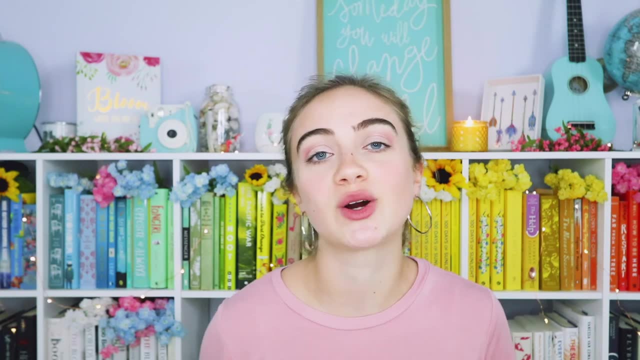 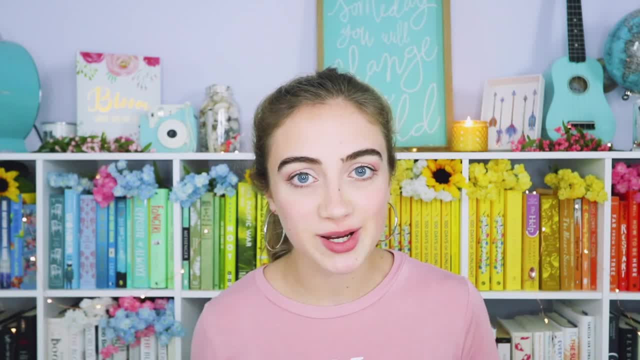 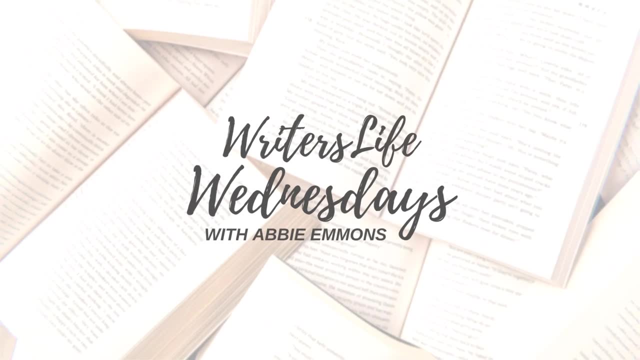 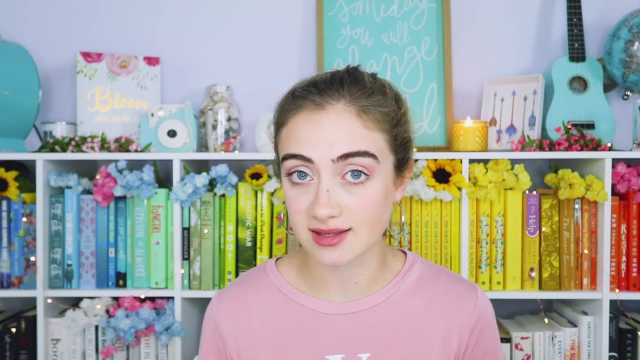 And that personally helped me so much. So grab a notebook and let's get started. Step one: choose your genre. I like to start with genre, because it feels like the easiest thing to figure out. What genre do you gravitate towards reading? That's probably the genre that you should. 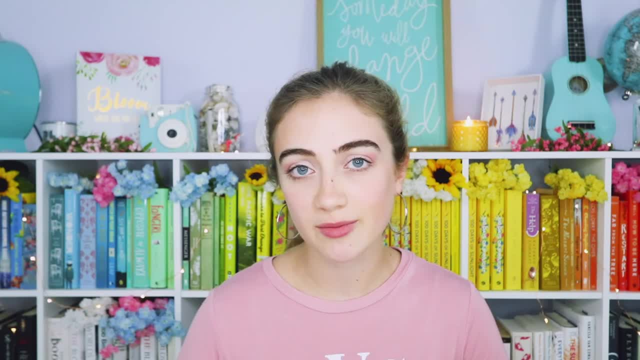 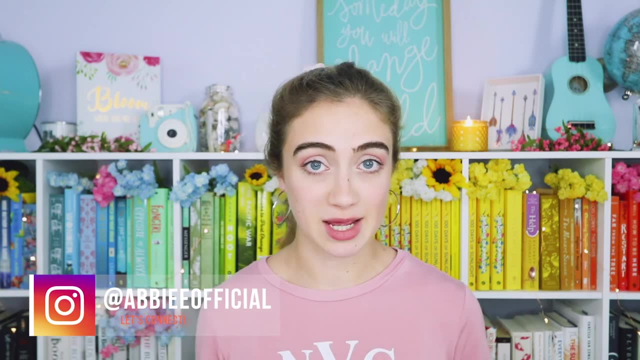 write in. Chances are this is the genre that you've already been thinking about writing in, but not always. I know that for myself, the book ideas that develop the quickest and easiest are contemporary in the contemporary genre, because that's mostly what I read, Not that. 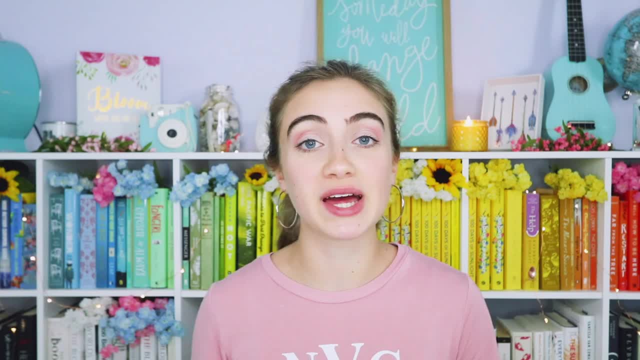 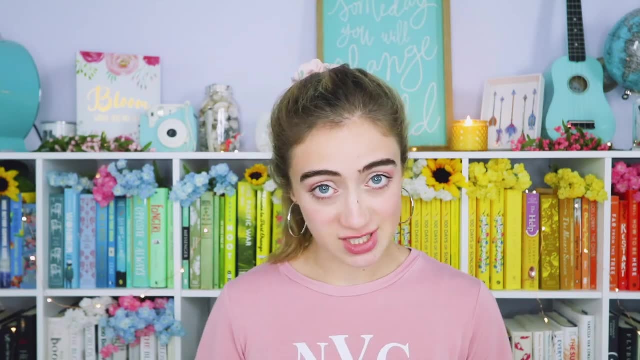 I can't write other genres. not that you can't write other genres, but it's best to stick with what you know and what you're comfortable with, especially if you're new to storytelling. The cool thing about choosing a genre is that it automatically narrows your options way down. Let's 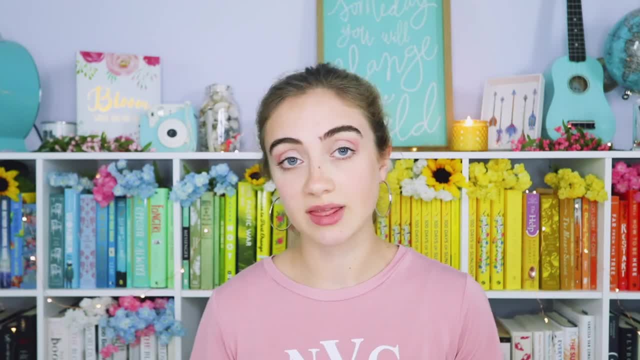 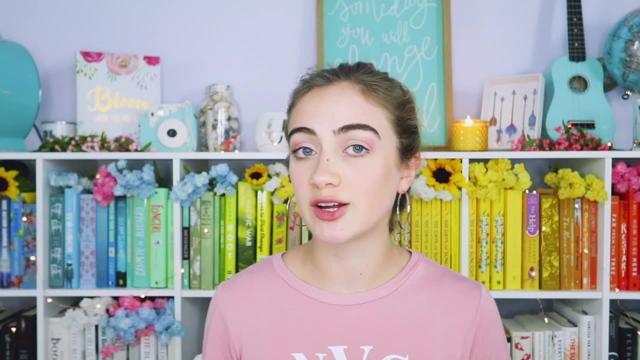 say: you know you want to write a contemporary romance. Well, knowing that is really helpful because it keeps you away from writing a psychological thriller or a fantasy, and vice versa. So once you've got your genre, let's move on to step two: Find your theme. We talked about theme. 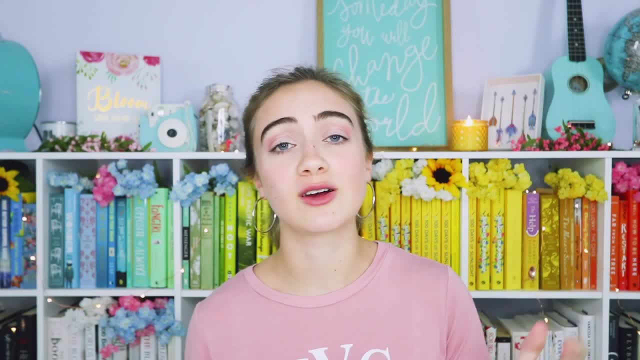 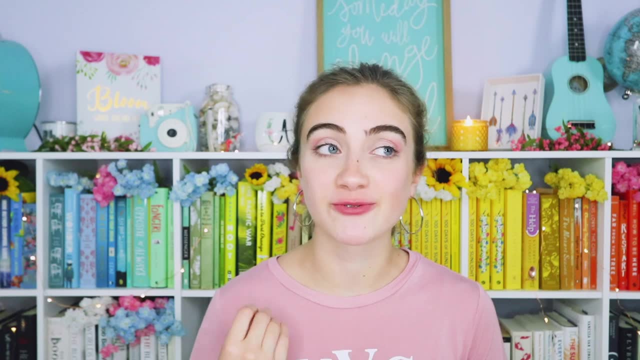 in depth, super in depth last week. Check out that video if you haven't seen it already. but in a nutshell, theme can be defined as the truth. you want to scream from the rooftops And for me it's always the first question I ask myself about a story idea. What is the theme? 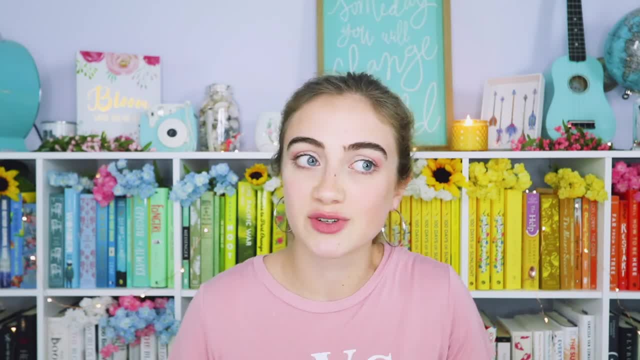 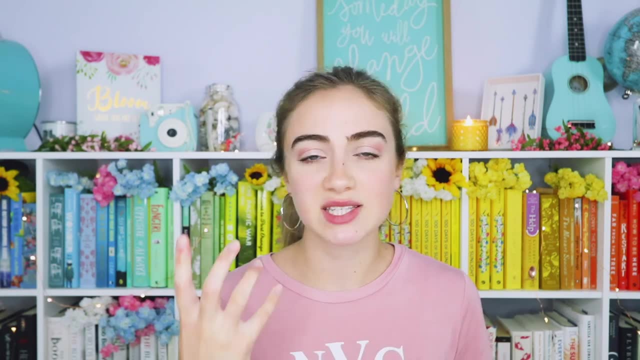 Because without a theme, your story doesn't really matter. And if your story doesn't really matter, what's the point in writing it? But I know that you have a passion for a truth burning inside of you And that's part of the 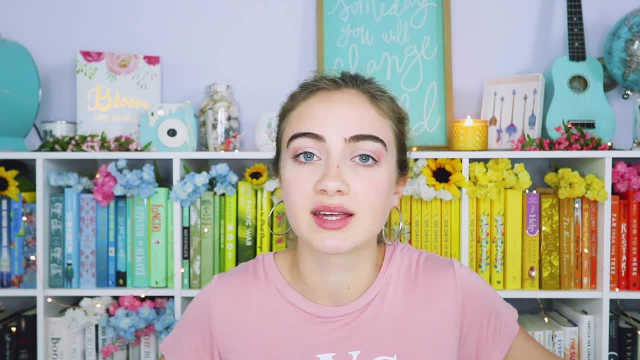 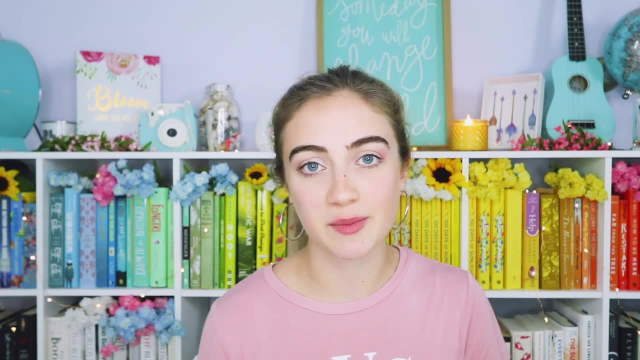 reason why you even want to jump into this whole crazy storytelling thing to begin with, because something's calling you to pick up a pen and connect with the human heart. There is a theme that you're passionate about writing into your story, whether you know what. 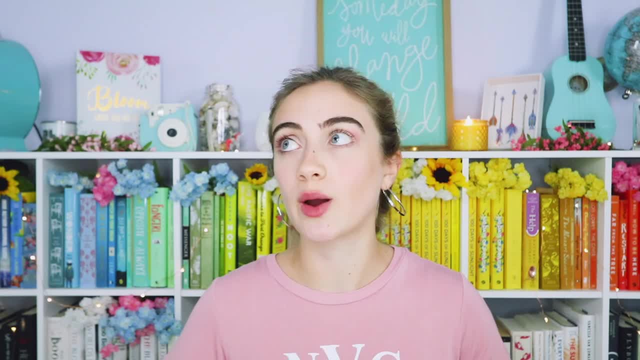 it is yet, or not. So ask yourself: what is the truth? I want to scream from the rooftops. What is the truth that my protagonist is going to learn over the course of their internal journey in the story and inadvertently teach it to me? And that's what I'm going to talk about today. I'm going to 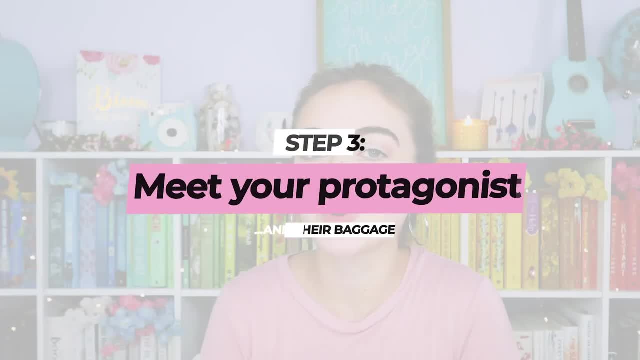 talk about the theme that you're passionate about writing into your story, whether you know what it is yet or not. So ask yourself: what is the truth? I want to scream from the rooftops. What is the truth that my protagonist is going to teach the audience? Step three: meet your protagonist and their baggage. 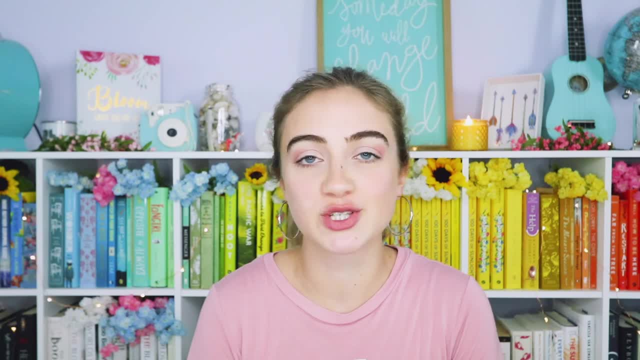 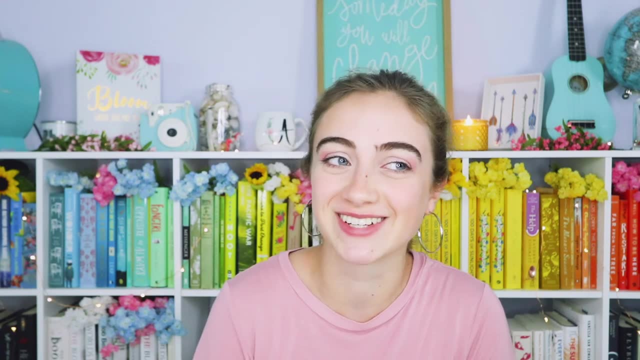 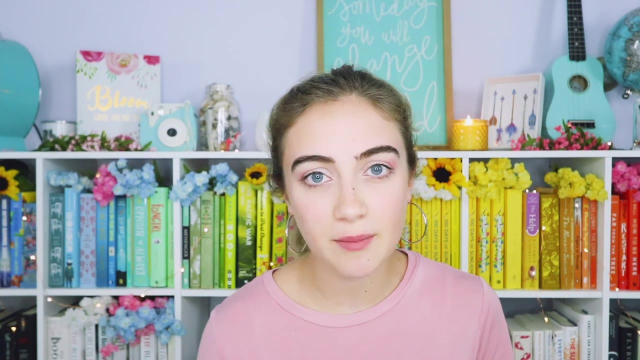 Characters are the most important part of storytelling. Why? Because story isn't about what happens. It's about how what happens affects and transforms the characters. I can never say that enough. If you can make your reader fall in love with your characters and relate to them, they will want to read. 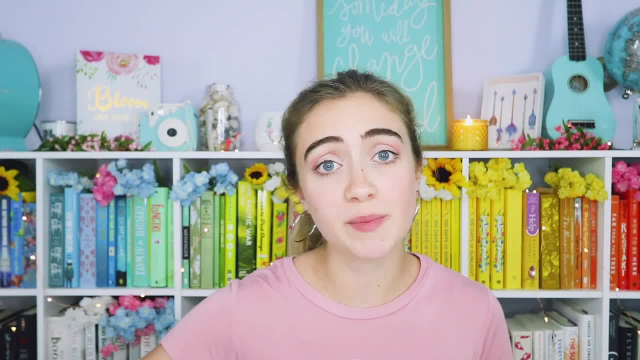 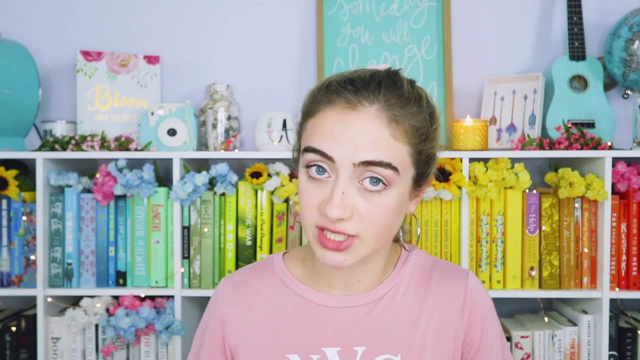 everything that happens to these characters, whether it's a trip to Starbucks or a voyage across the galaxy, And that's why, before you start doing anything with your plot, you need to meet your protagonist. This is just going to be a rough outline, so you don't need 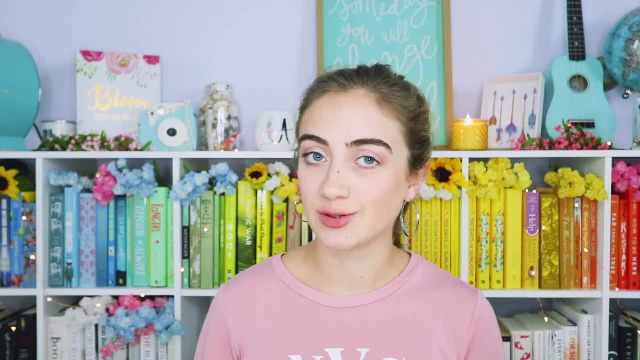 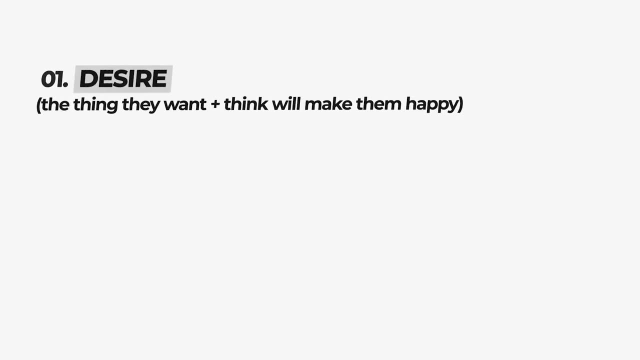 to dive too deep into developing your protagonist yet, But you should figure out a few basic things that will hugely impact the story. One: their desire. the thing they want and think will make them happy. Two: their fear, the thing stopping them from going after the thing that will make. 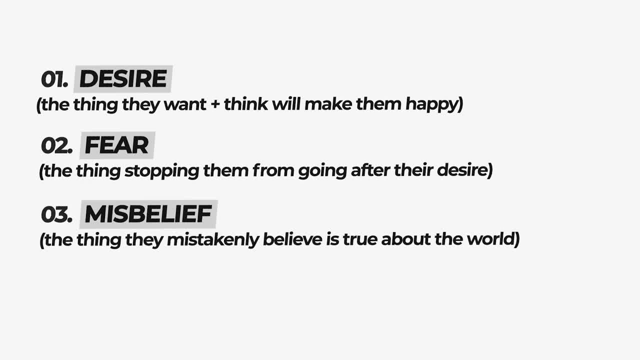 them happy And three their misbelief: the thing they mistakenly believe is true about the world, which is the exact opposite of what they think is true about the world, which is the exact opposite of your theme. So flip your truthful theme on its head and make it a lie. Boom. 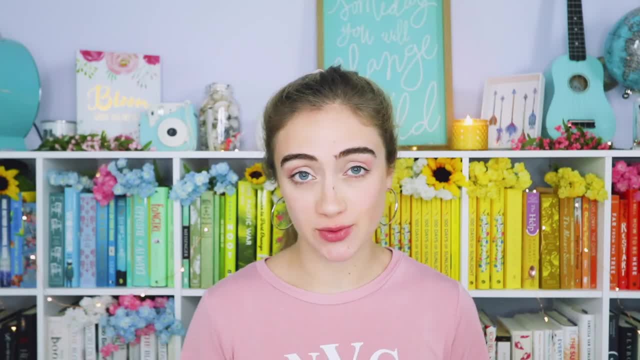 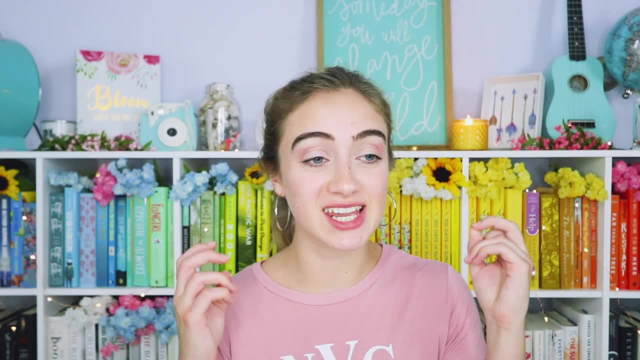 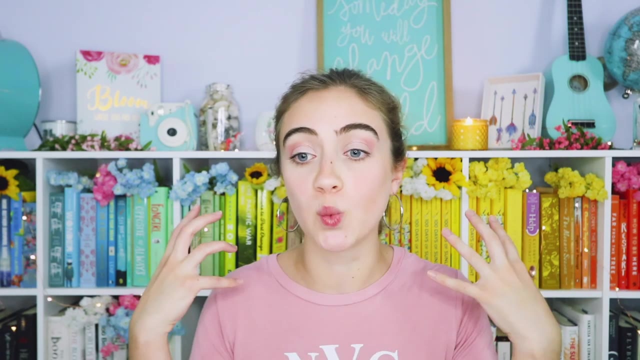 that's your protagonist's misbelief. These are always the first three things that I sketch for my protagonist when I start plotting a novel, And it's amazing what this process does. It takes an otherwise two-dimensional character and makes them this incredibly dynamic, conflicted person that you want to be a part of their life. 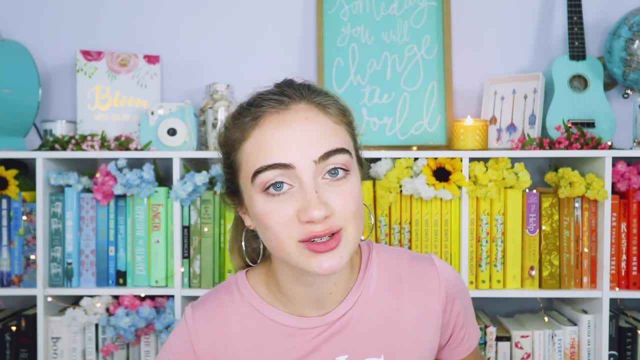 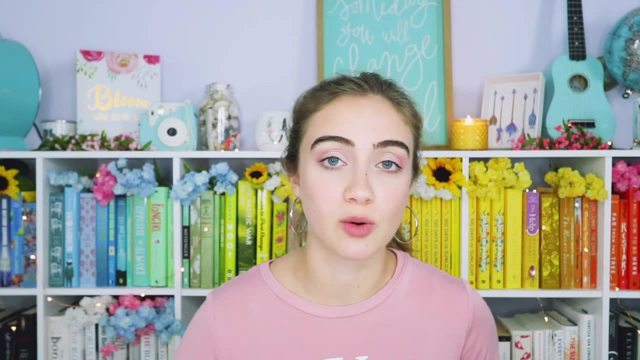 See, this is the thing that your reader's brain is subconsciously searching for: An internal journey leading to an aha moment which will put to death a misbelief that your protagonist has held onto their whole life. Creating characters is the biggest and most important part of 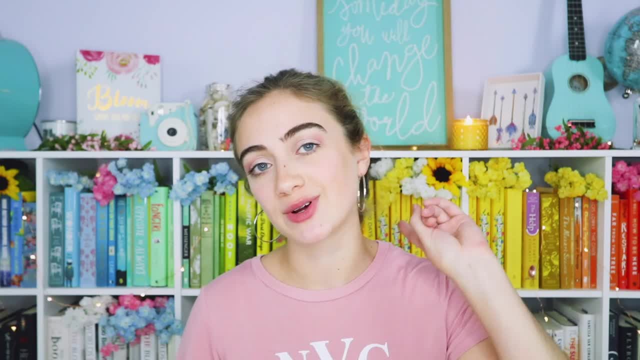 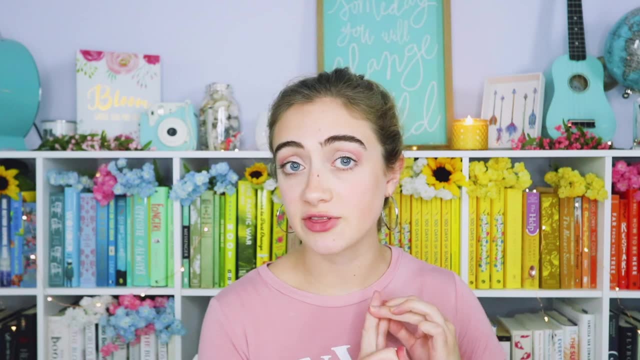 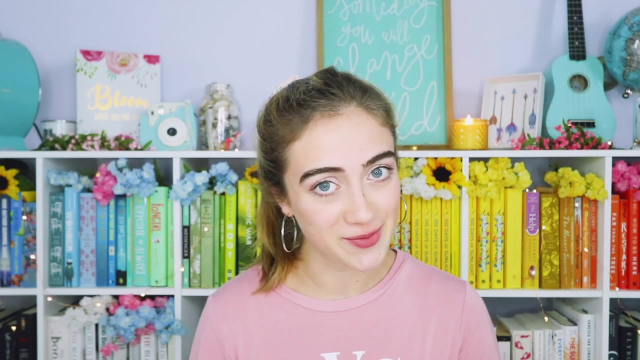 storytelling. So definitely take your time here- Don't rush- And also check out my character creation videos. Okay, so now we know three major things about your story: the genre, the theme and your main character and their baggage. That's a lot going on, but let's take it one step further. 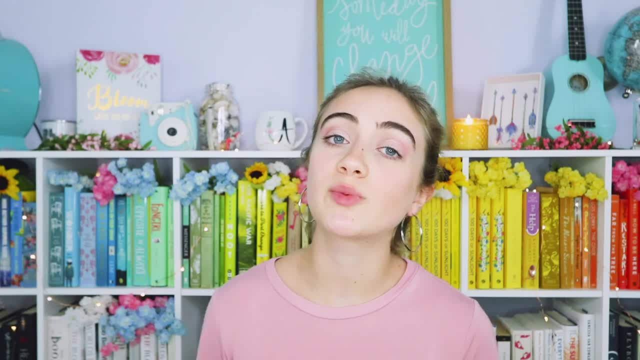 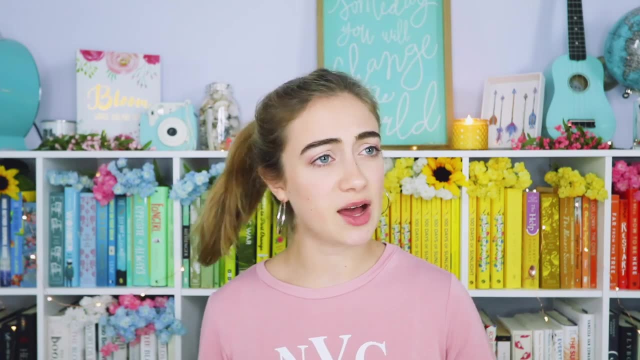 Step four: describe your vibe. Choose three words that describe the vibe of the story you want to write: Mysterious, thrilling, suspenseful, cute, sad, happy, badass, heartwarming, dreamy, et cetera. I love doing this. 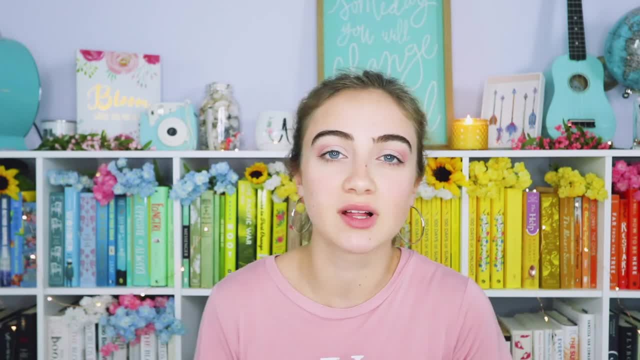 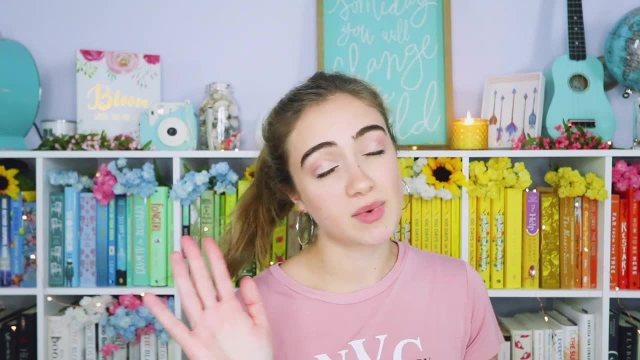 because it helps me get a basic idea of how I want to feel writing this story. What is the mood, the emotion that you want your readers to feel while they're reading this story? Remember, you can keep it super vague, So write down your three words, or you can do more than three if 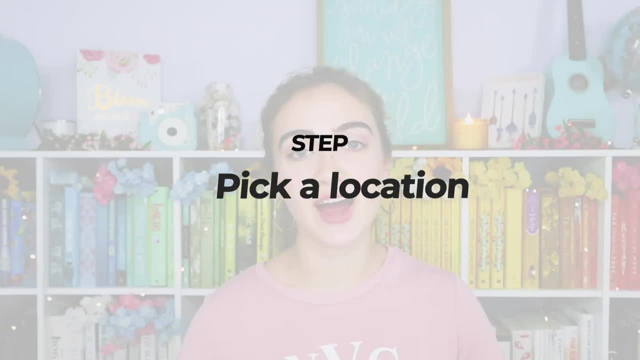 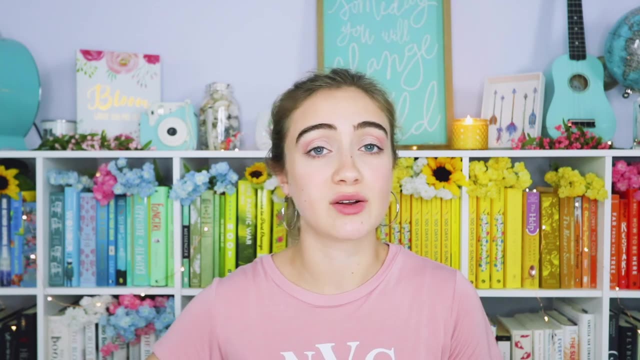 you want And let's move on. Let's move on to the last step, Step five: pick a location. This kind of circles back to step one when we talked about genre. Obviously, if you picked a genre like science fiction or fantasy, 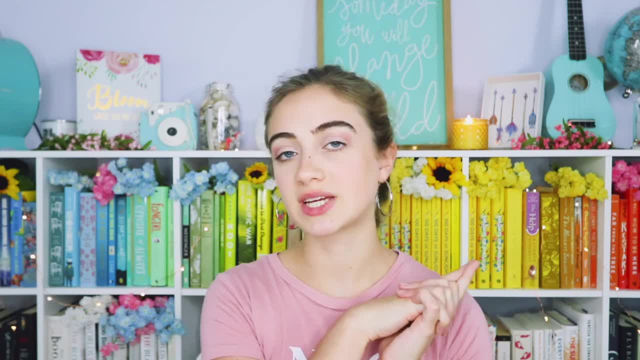 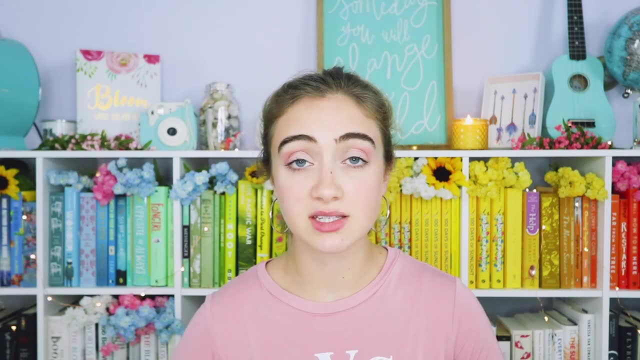 you'll be setting your story in a fictional location. If you picked contemporary or any kind of story that exists in the real world, then you'll want to figure out what part of the world best suits the vibe that you just described a minute ago. Or you can always just throw a dart. 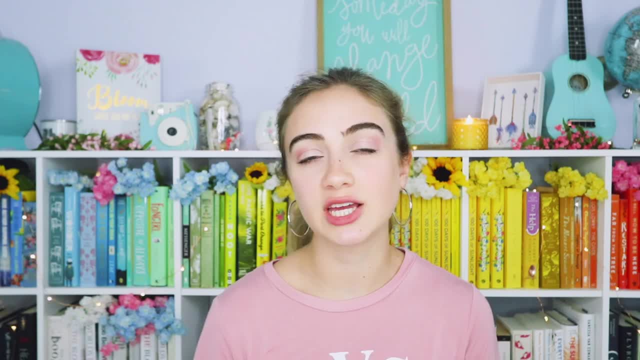 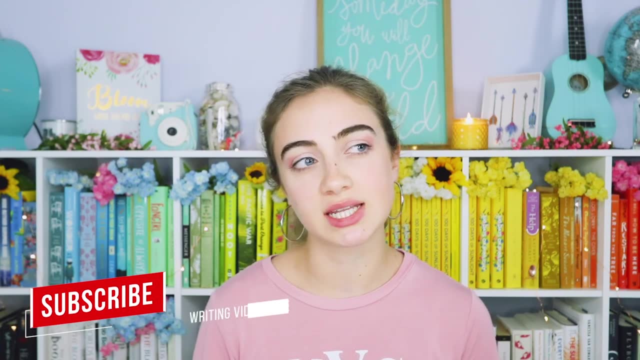 at a map. whatever works Picking a location. Picking a location will not only help you to zone in on what your character's world is like, but it will also help you to understand how the location is going to affect your character's. 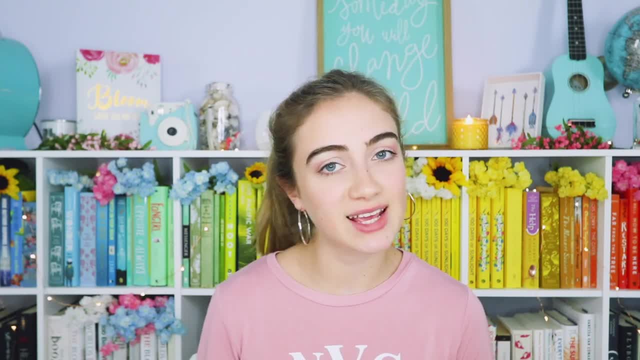 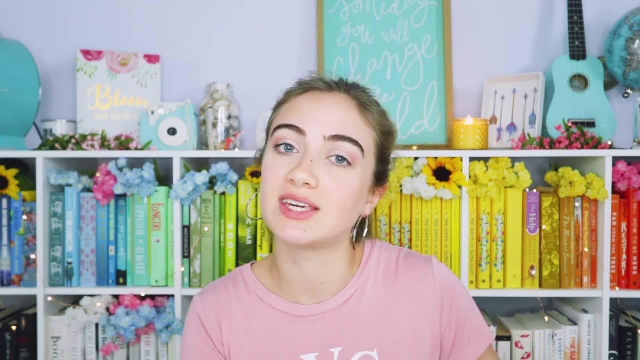 internal journey. Of course, your character conflict can adapt to any environment. For example, your power hungry protagonist could be queen of a fantasy land, or she could be CEO of a major corporation in the real world, But it's good to know your genre and location from. 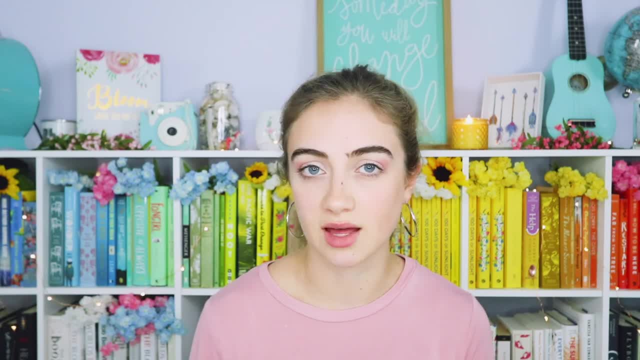 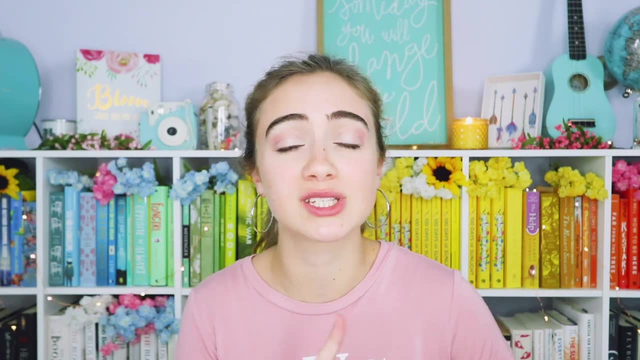 the outset, or else you won't really know what kind of story you're telling. So boom. that's the five step process. but I'm not done yet. I have a few bonus tips that will 10X your inspiration. But first I just want to say you don't have to do all five of these. 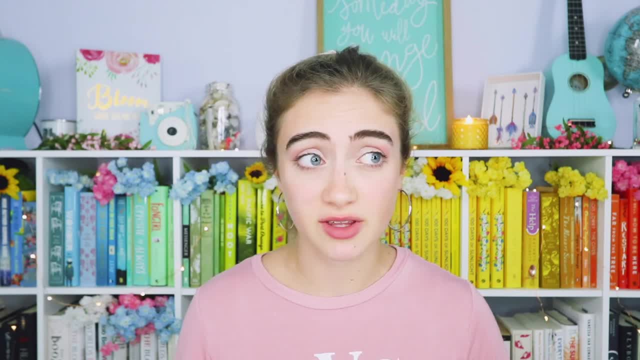 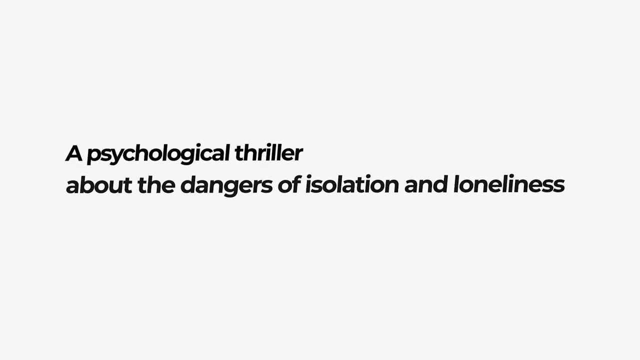 things from the start. Three out of five, two out of five, even, is fine. For example, let's say we know we want to write a psychological thriller about the dangers of isolation and loneliness- Great, That's our genre and our theme. Or let's say we know we want to write about a 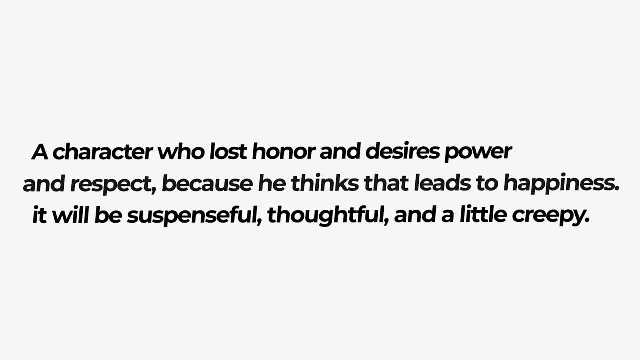 character who lost honor and desires power and respect because he believes that leads to happiness. the story is suspenseful, thoughtful and a little creepy. Great. That's our protagonist's conflict and the vibe. Or let's say we know that we want to write a cute contemporary. 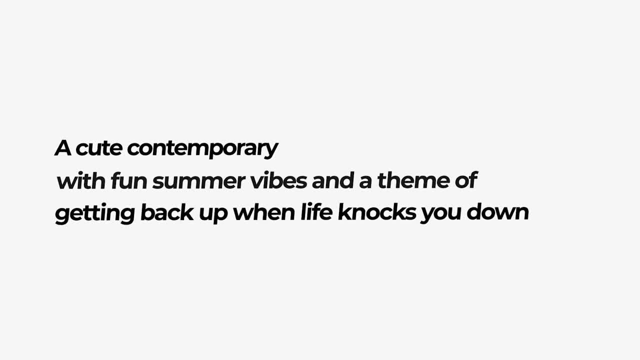 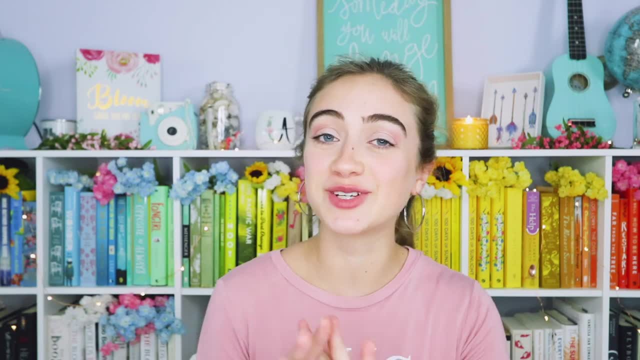 with fun summer vibes and a theme of getting back up when life knocks you down. That's- oh wait, that's 100 days of sunlight. Shameless plug. Okay, but seriously, you don't need all five. Three out of five, two out of five is great. Just remember that. 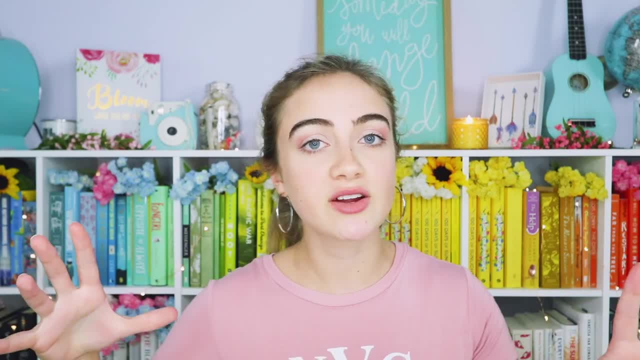 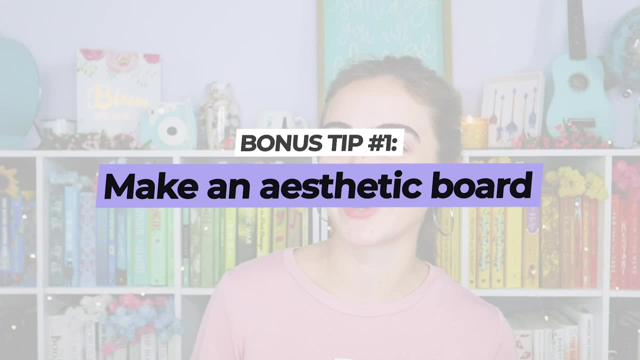 the more questions you answer, the closer you get to having a clear idea of the story You want to write. Now time for bonus tips. Bonus tip number one: make an aesthetic board. If you've been around here for a while, you might know I'm obsessed with making. 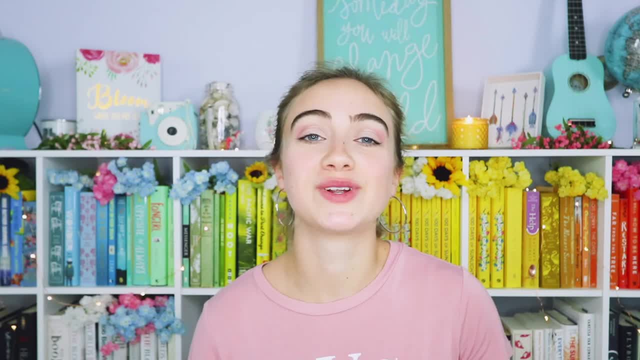 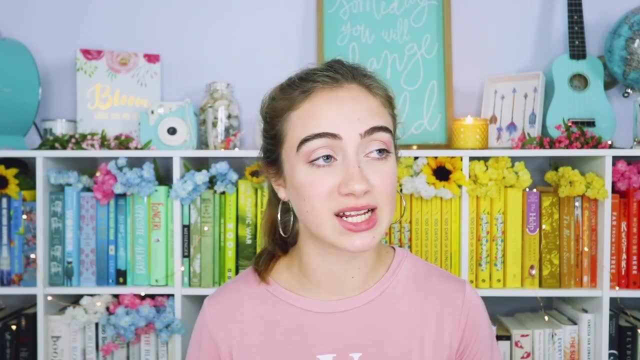 aesthetic boards for my books on Pinterest. It's actually one of the first things I do after I get a new story idea: Drop everything and immediately start building an aesthetic board, and it just makes me want to write the story so much more. This is a lot like figuring out. 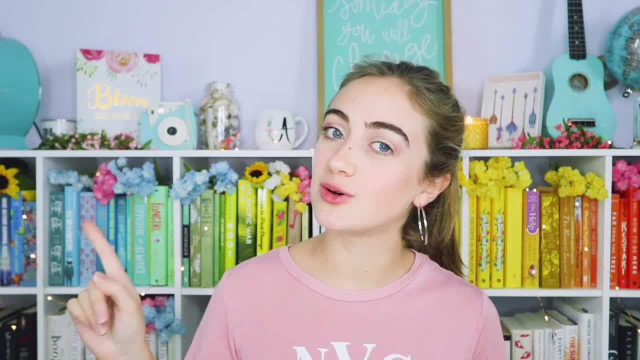 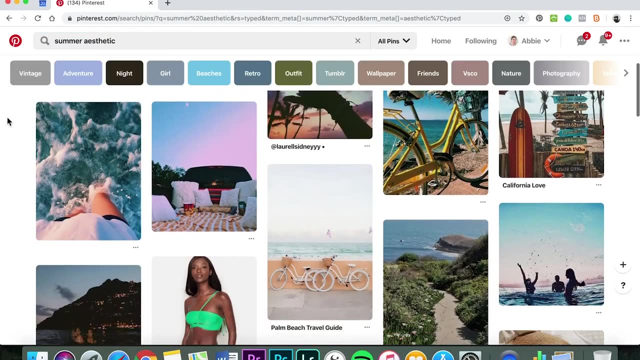 your vibe. In fact, you can use those vibe words that you chose a little while ago when you're building your aesthetic board. Search them in Pinterest and put the word aesthetic after it. Guaranteed you will find so many visuals that will inspire you for your story. 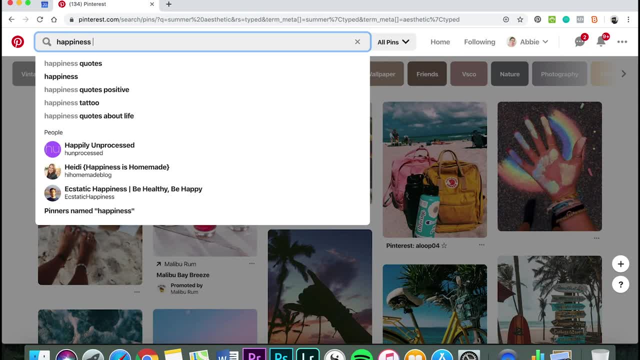 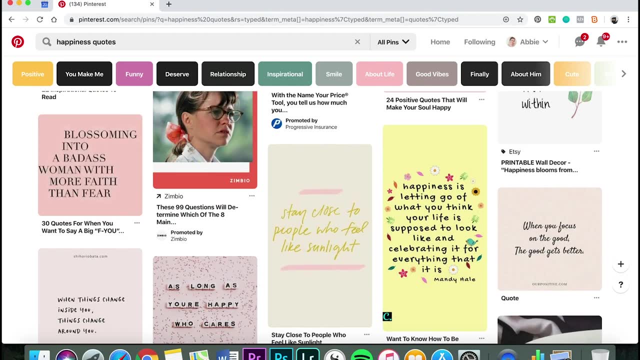 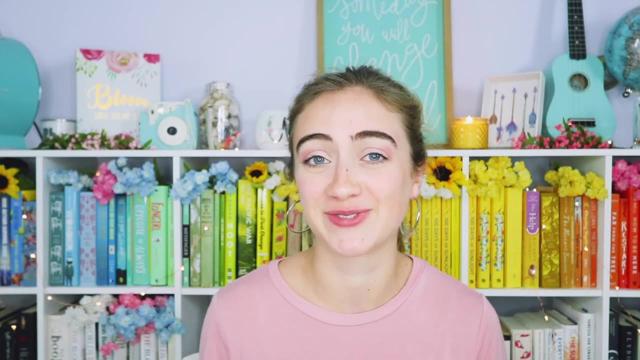 Also, you can search your theme keywords like happiness, loneliness, power, et cetera, and put the word quotes after it. Boom, You have all kinds of inspirational words to drive home the point of your theme, mixed in with your aesthetic photos. Oh my gosh, it's just so much. 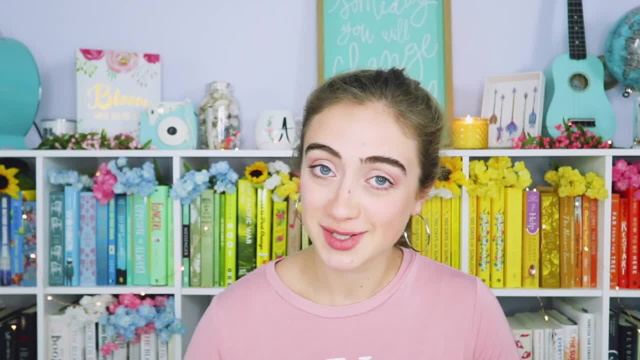 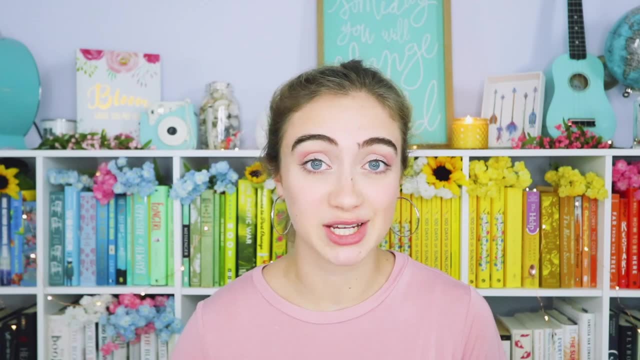 fun. I could literally do this all day, So if you're anything like me, don't get carried away with this Bonus. tip number two: make a playlist. This is another thing that I do pretty much immediately after getting a new story idea. 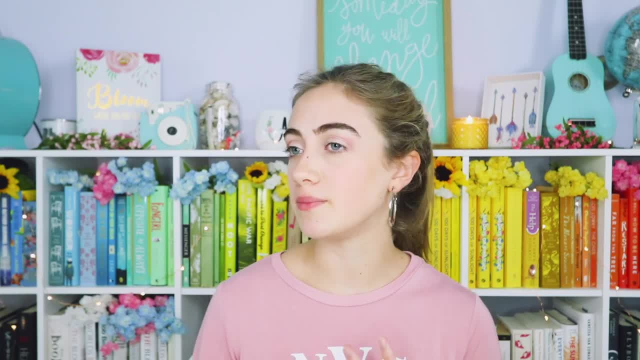 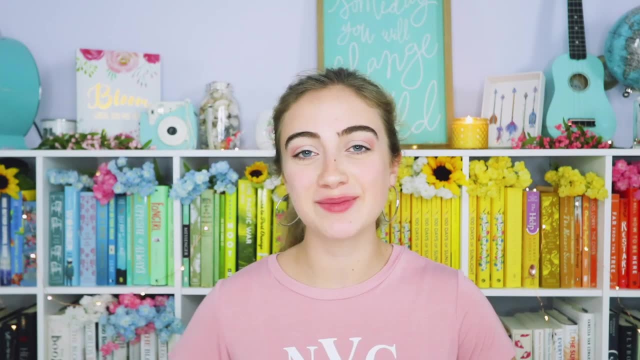 The genre and vibe of my story will have a big influence on what music reminds me of this story. Plus, the message of certain songs might align with my theme. Basically, any songs, any music that reminds me of my book goes on its own curated playlist I am totally obsessed with. 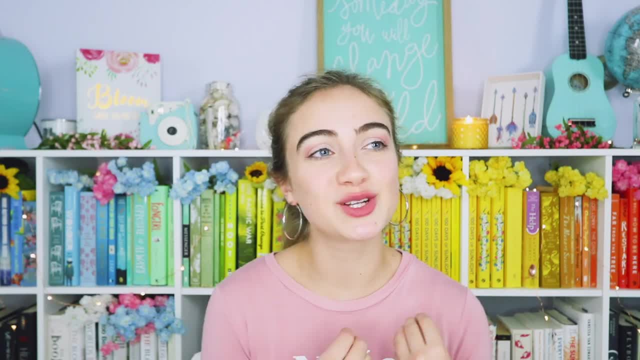 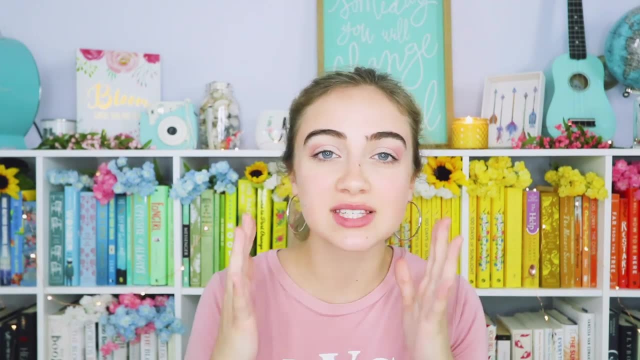 music, not just because it's awesome in general, but because it plays on your emotions and makes you feel like you're in the right place. So if you're in the right place, you're in the right place to feel, And this emotion can really fill in the gaps of your story idea. It's not even like 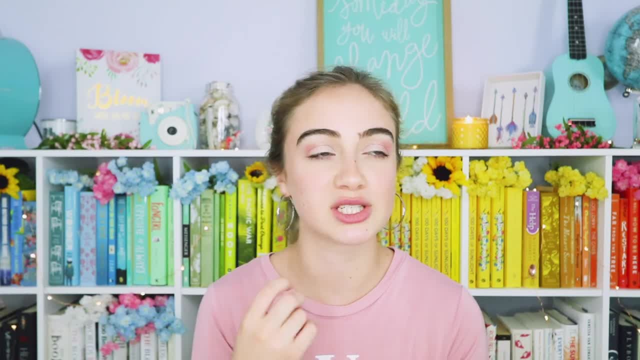 something I can explain, but when I listen to music that reminds me of my book and I just imagine the characters and the story and I just experience the emotions that they're feeling and let the music touch my soul, It's just like it's a visceral experience I can't even describe. 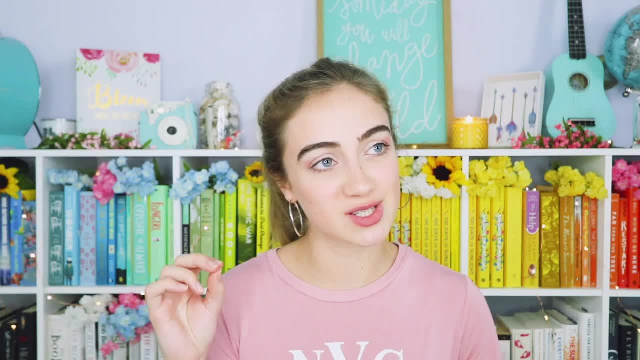 Also, it's awesome to listen to instrumentals that you can sort of just like make the soundtrack mentally. imagine it to be the soundtrack of certain songs that you're listening to. So if you're listening to music that reminds me of my book, 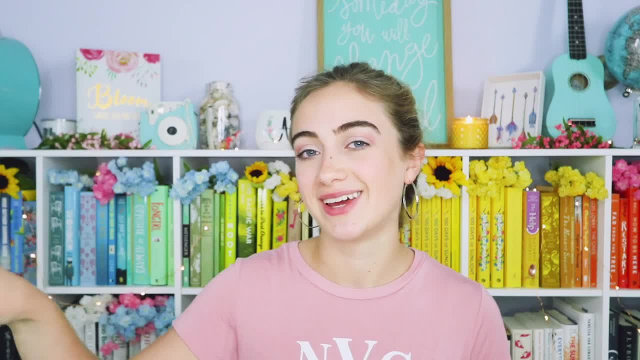 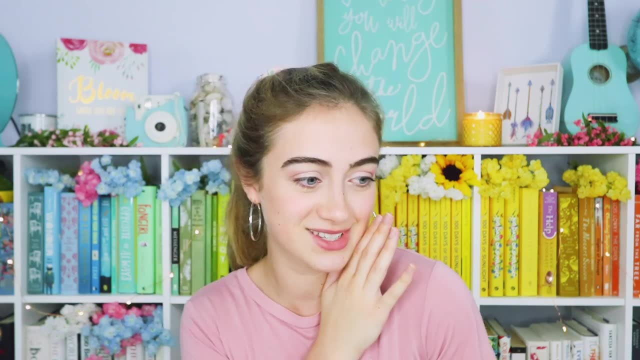 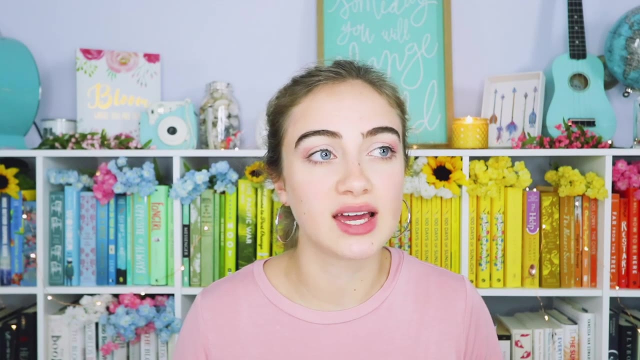 I do that all the time And those go on a separate playlist. of course, that is like the soundtrack. Sorry, I stole my soundtrack from everybody else's soundtracks. It's awesome. Bonus tip number three: give it a working title. Don't just go around referencing your story idea. 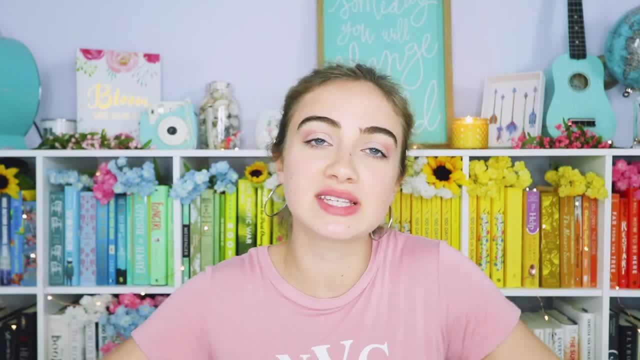 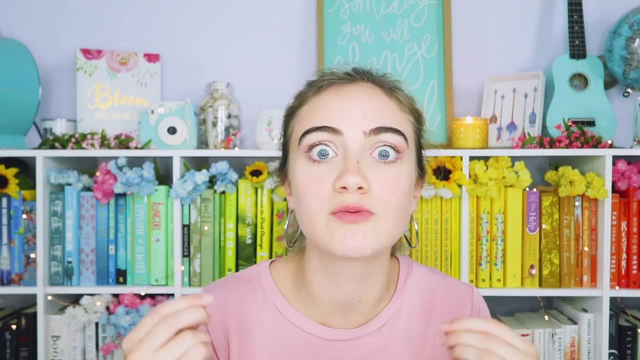 as my story idea. It's just it makes it sound so illegitimate and it just like an idea. It's more than that. I mean, you're excited about it, You're passionate about it, You're going to write it. So 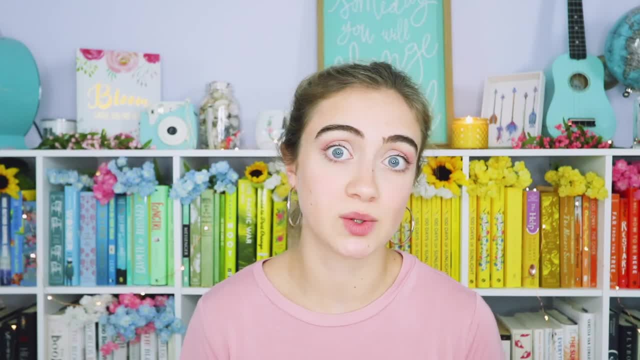 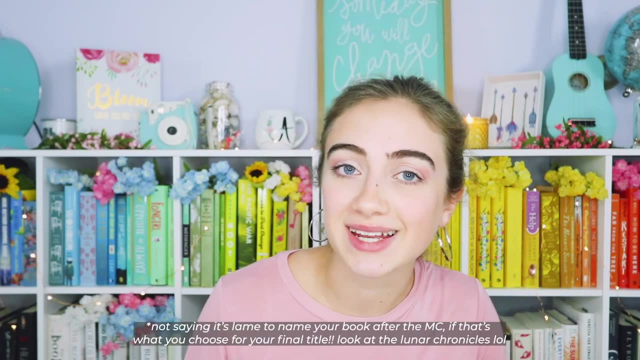 like it's already a book. give it a working title and it will feel more real to you, Even if it's nowhere near what the book is actually going to be called, Even if it's something really lame like the first name of the main character. I always used to do that with my stories up until, like 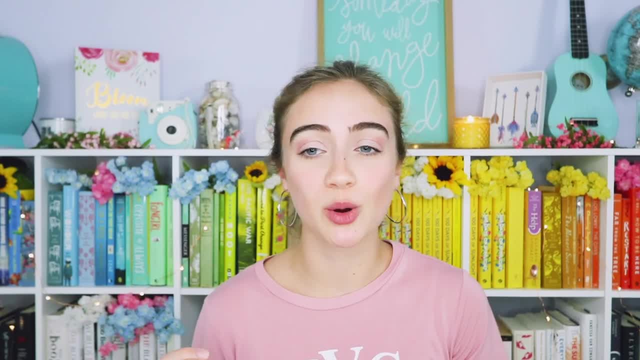 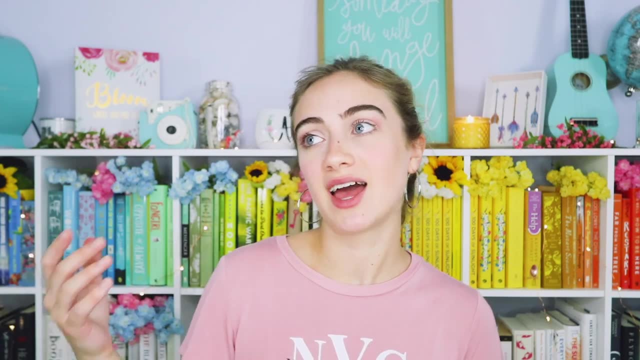 a few years ago. But seriously, a working title just makes me so much more excited to write a story and make my idea a reality. So, boom, that's it: How to come up with a story idea out of thin air. Let's recap that five step process from before. 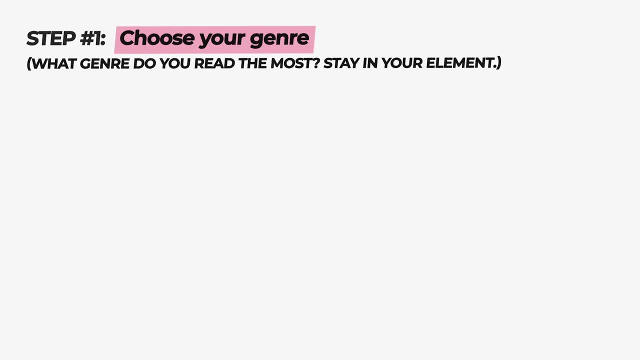 Step one: choose your genre. What genre do you read the most? Stay in your element. Step two: find your theme. What is the truth you want to scream from the rooftops? Step three: meet your protagonist. What is their desire? fear and misbelief.